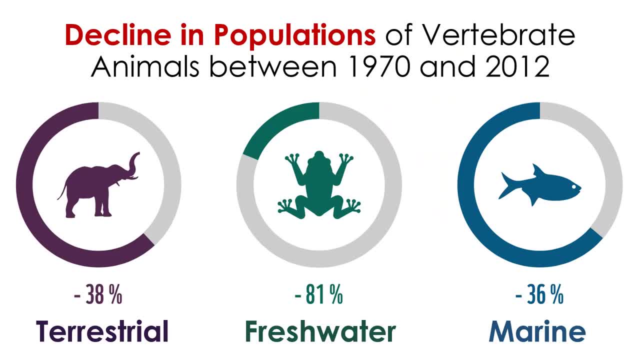 well. Scholars have observed that many populations of vertebrate animals have vanished over the past few decades. Since 1970, populations of freshwater animals have declined in abundance by 81%. Terrestrial and marine populations have declined in abundance by nearly a third over that time. Currently, 41% of 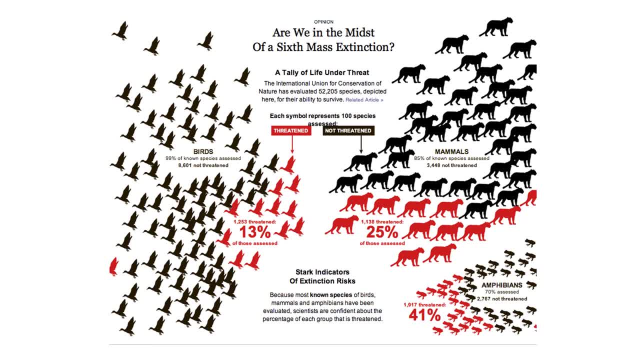 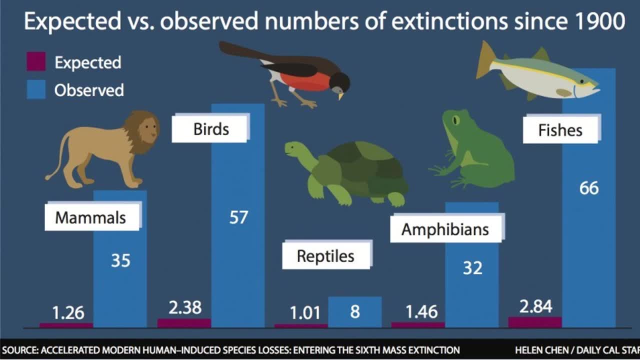 amphibian species are threatened with extinction, along with 25% of mammals and 13% of birds. Other groups of organisms face the same threat. It is clear, then, that the disappearance of species is not the end of the world, but rather the beginning of a new era. This is the beginning of a new era. 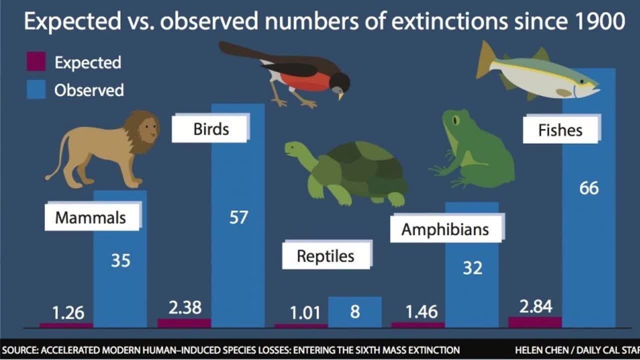 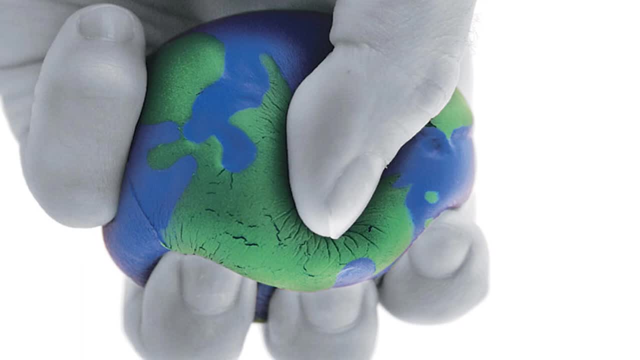 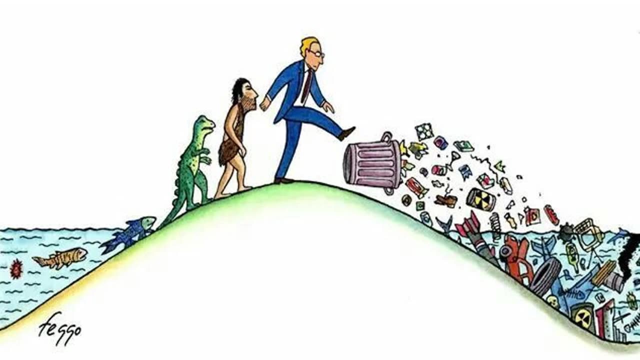 This is the beginning of a new era. This is the beginning of a new era is a very real and very concerning trend. all of the evidence suggests that life on Earth now faces an unprecedented crisis, one that is unparalleled in human history. this crisis is probably a consequence of multiple causes, but any 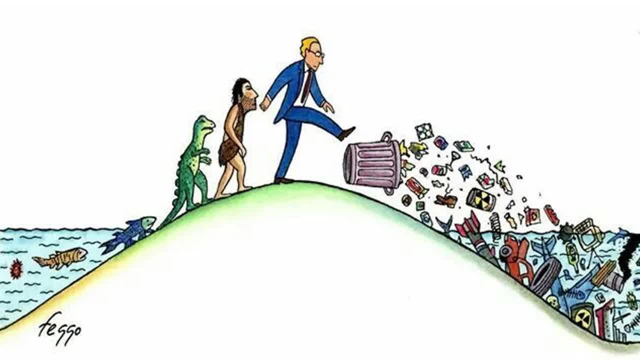 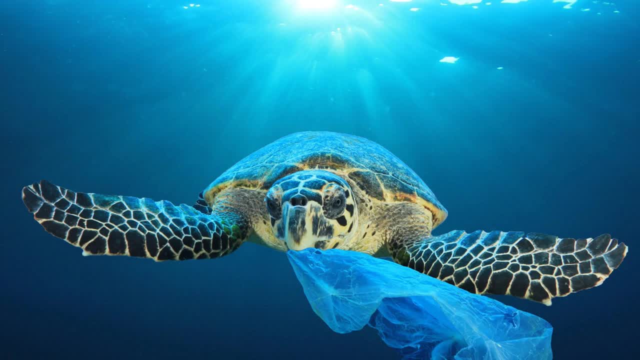 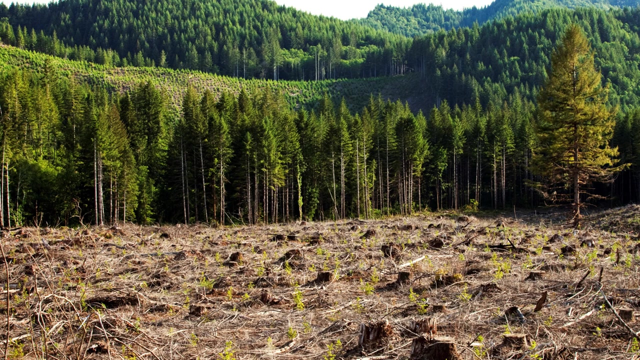 way you look at it, humans must be part of the problem. we produce garbage, waste, litter and pollution that are harmful not just to ourselves, but also to the other forms of life that share our planet. We cut down forests, develop coastlines, bury wetlands and destroy habitats that provide homes to countless. 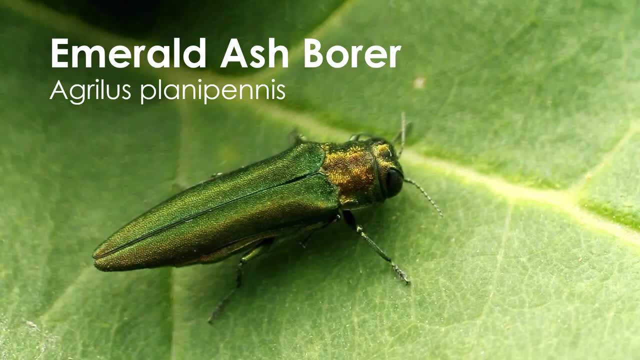 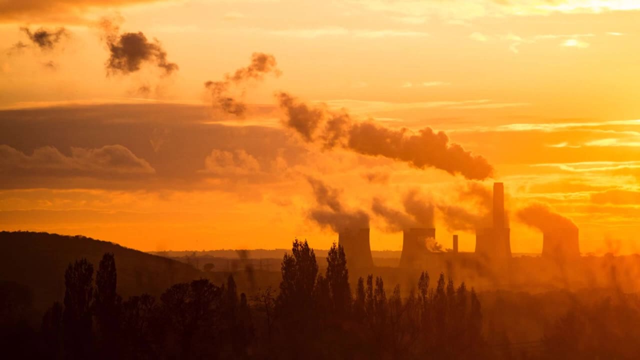 other species. We play a key role in spreading invasive species and other pests which wreak havoc on native populations around the world, And, of course, we produce an astounding amount of greenhouse gas that has the power to cause climate change and fundamentally alter all ecosystems on Earth. Humans may 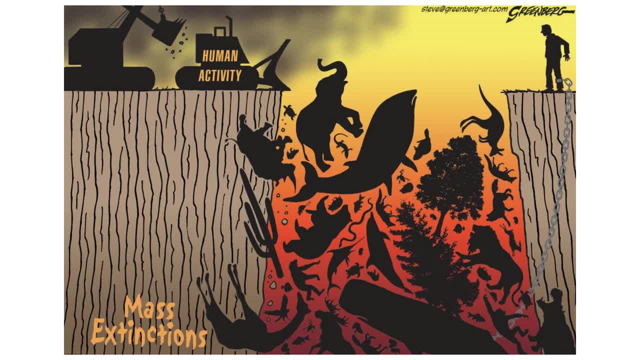 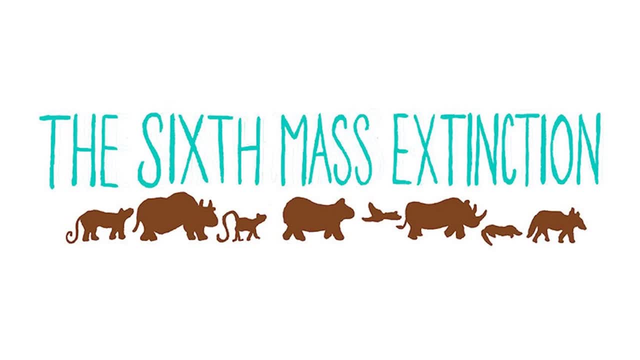 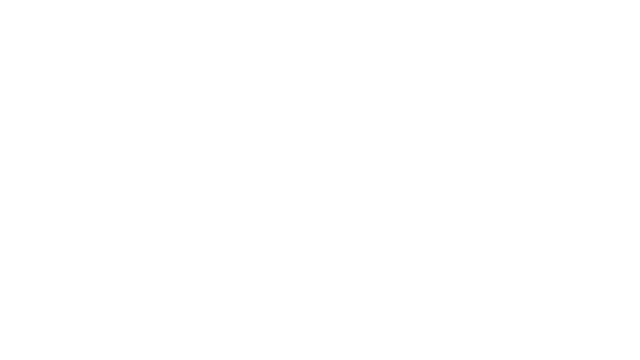 very well be the cause of this mass extinction. This crisis is being called the sixth mass extinction because there have been five similar events in the history of life on Earth. But what were the mass extinctions? How do we know about them? What caused them And what can they tell? 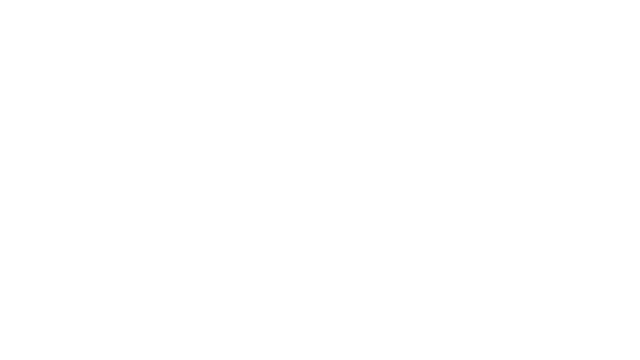 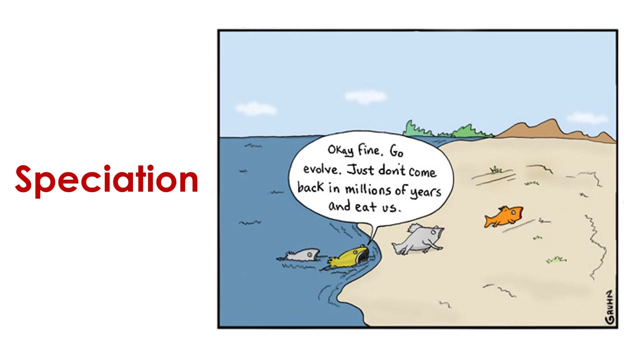 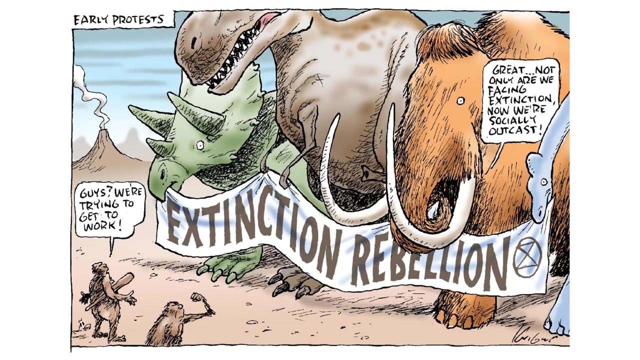 us about the current biodiversity crisis that we are facing. Species originate on our planet through a process called speciation. Populations of organisms evolve new traits and diverge from their ancestors over time, becoming increasingly different and unique. Extinction is the flip side of 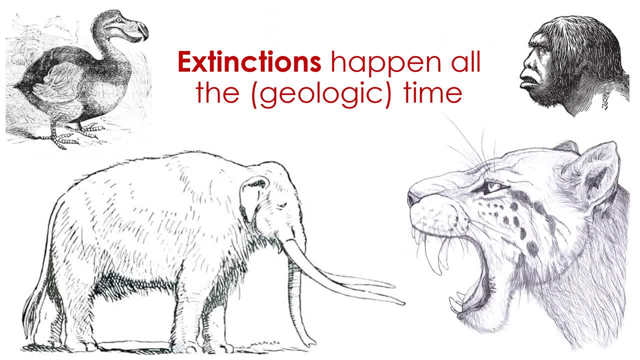 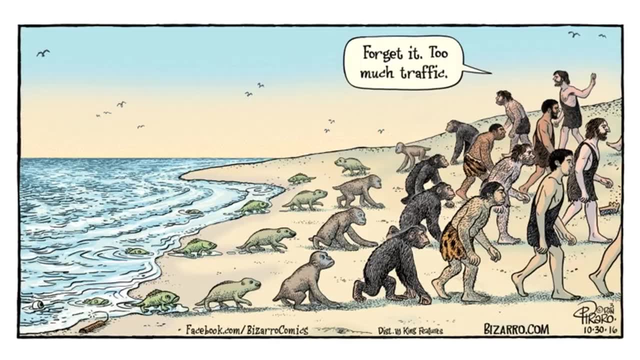 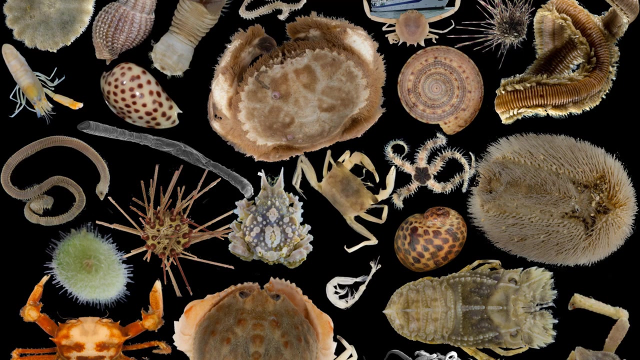 the coin. As we have observed over the past 500 years, species disappear all the time. It's important to recognize that speciation and extinction are natural processes on our planet. At some point, all species on our planet disappear. Some species go extinct not long after their origination, while others have survived on. 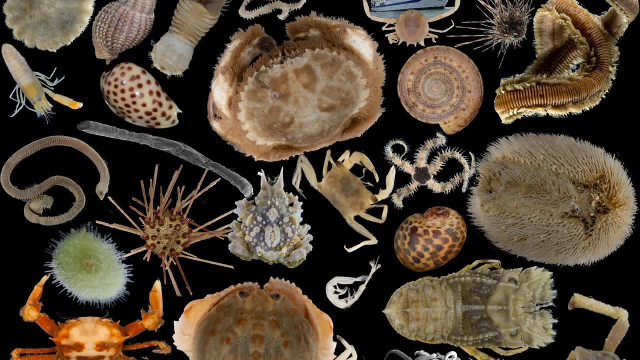 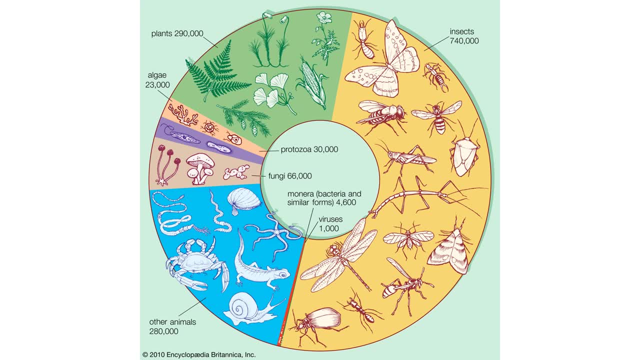 Earth for hundreds of millions of years. Scientists have identified over 1.4 million species on Earth, And some researchers estimate that there could be anywhere between 3 million and 30 million species of plants, animals, fungi, protists and prokaryotes overall. 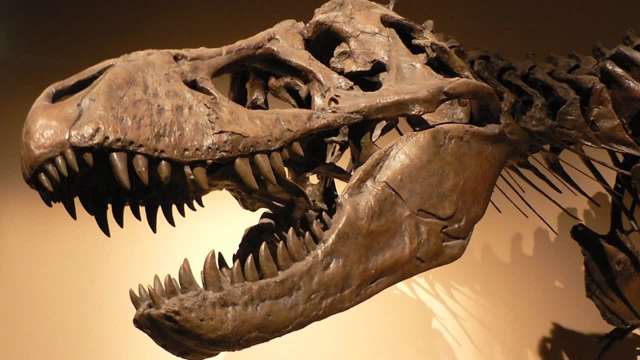 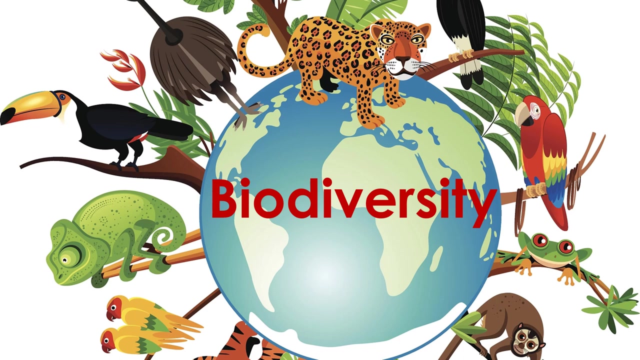 Paleontologists so far have discovered more than 250,000 species in the fossil record. Many of these species are extinct. The number of species that have ever existed on Earth may be astronomical. The number of species is directly related to biodiversity. Biodiversity is the variety of life on the world, or alternatively. 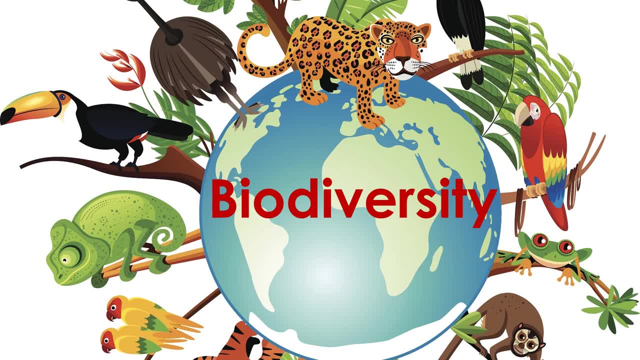 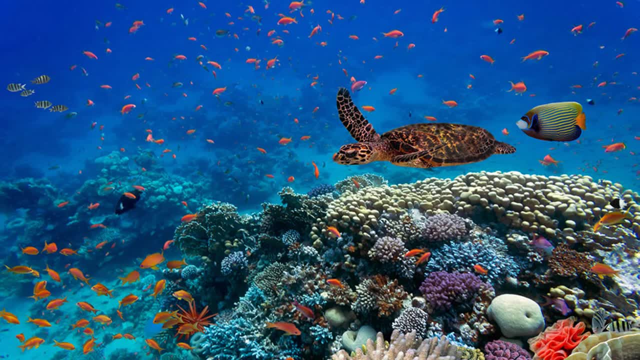 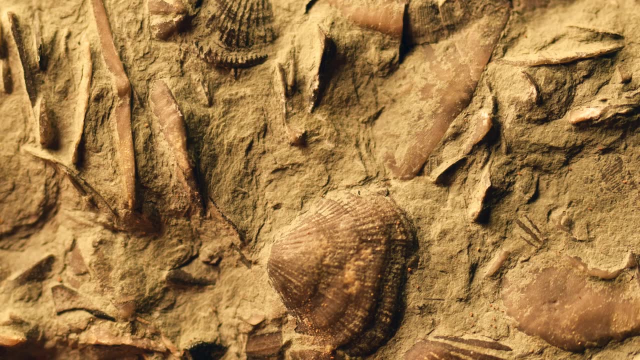 in a particular place or ecosystem. Counting taxa like species is one of the easiest ways to get a sense of biodiversity. This statement is particularly true in paleontology, geology, as species are often easy to identify but hard to understand, since they are no longer. 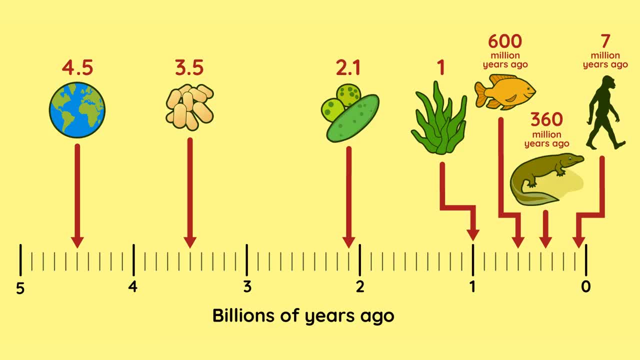 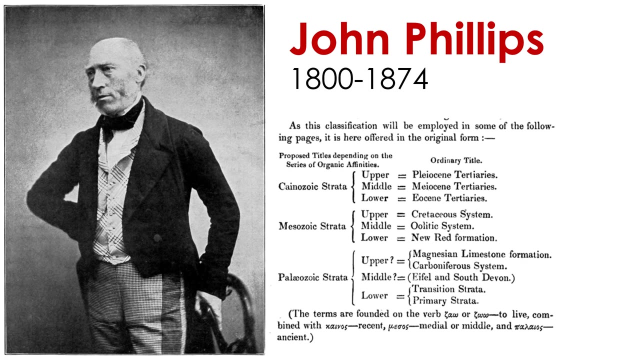 alive today. For centuries, paleontologists have wondered how the biodiversity of our planet has changed over time. One of the first geologists to tackle this question was John Phillips, the Englishman who developed and published the first global geologic timescale. 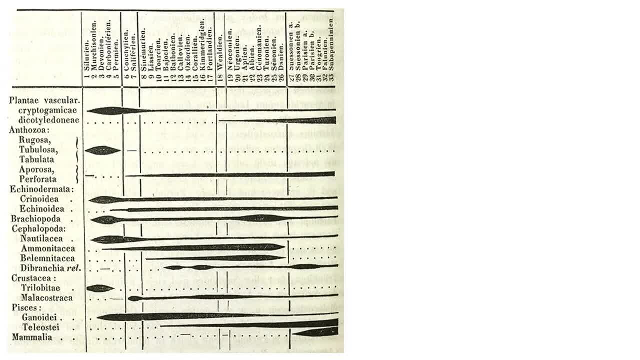 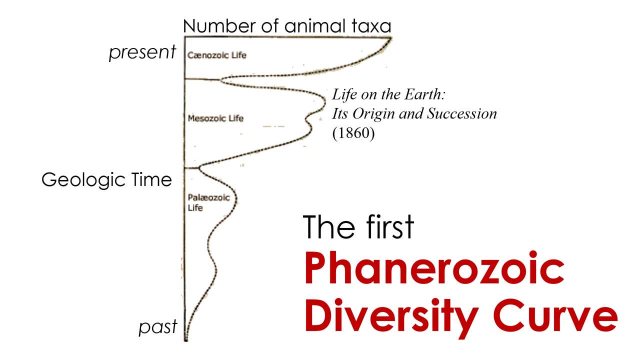 Phillips, of course, employed biostratigraphy to develop the geologic timescale. In the process, he studied the fossils that are unique to rocks of different ages. Using this knowledge, he produced the first Phanerozoic Diversity Curve. A Phanerozoic Diversity Curve is a geological study of the geological structure of a geological 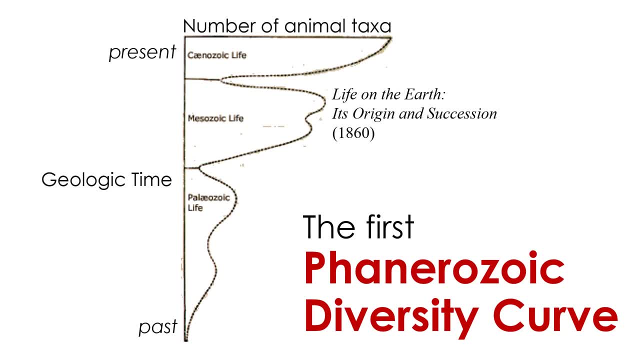 system. The Curve shows how Earth's biodiversity has changed over the last 541 million years, over the course of the Phanerozoic Eon. Biodiversity is represented on one axis by the number of taxa, such as the number of species, genera, families or orders. 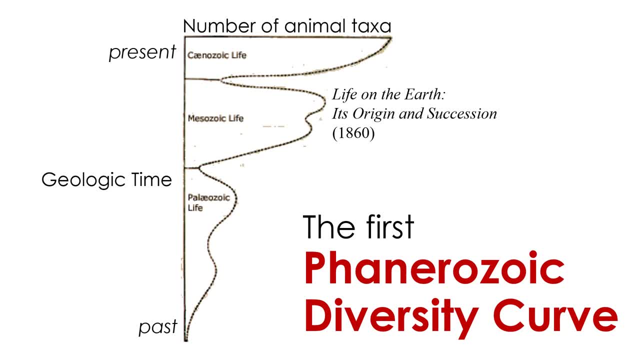 The other axis is geologic time, spanning from the past to the present, The new. We will discuss this in depth in a moment. Phillips's Diversity Curve was rudimentary at best. He basically guessed how many taxa existed at different times in Earth history, given. 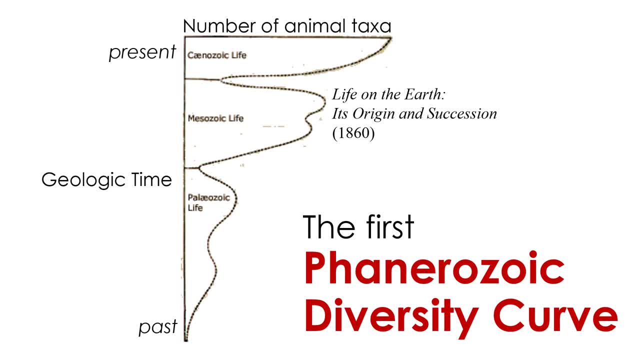 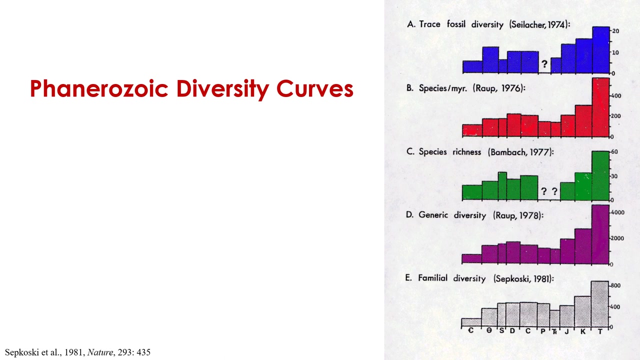 his extensive knowledge working on biostratigraphy. That said, the curve was intriguing- has increased over time. Life has been becoming increasingly more diverse since the beginning of the Phanerozoic. In the century following Philip's work, many paleontologists attempted to expand on his research, but their efforts were 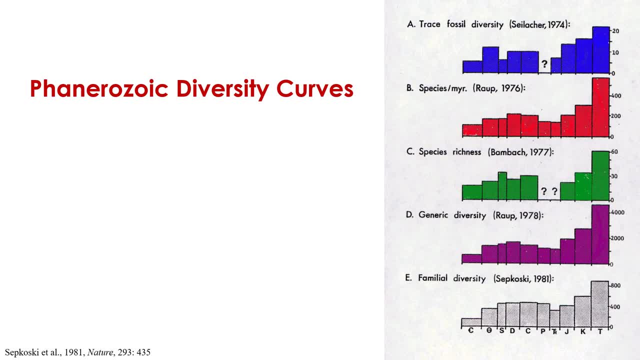 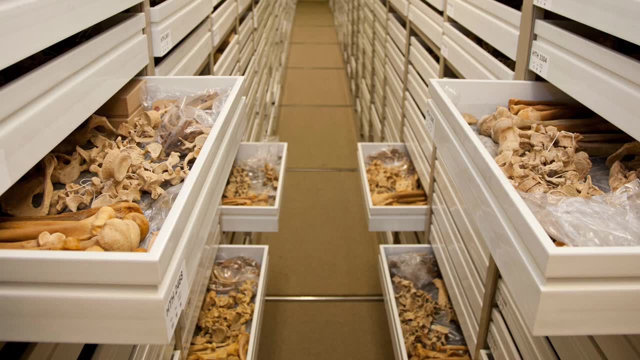 generally limited by the technology and resources at their disposal. In particular, they struggled to keep records of every taxon in the fossil record. Again, there are hundreds of thousands of species in the fossil record which have been reported from all around the world Prior to the advent of. 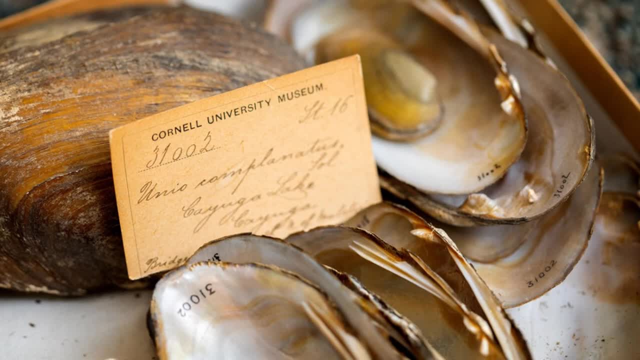 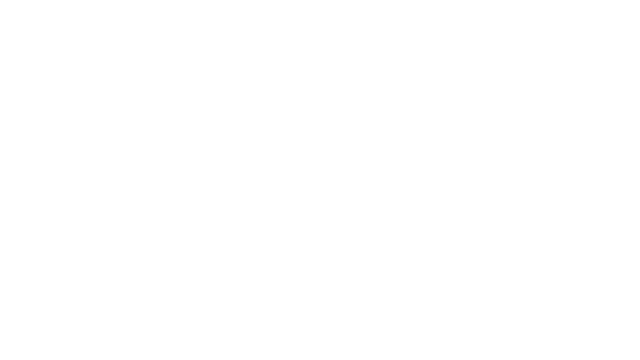 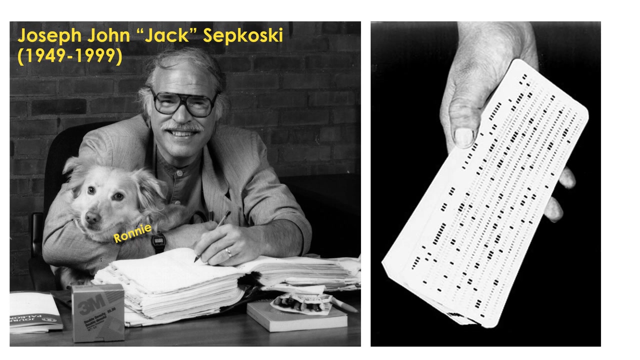 computing, it was virtually impossible for paleontologists to keep track of where every taxon came from. A breakthrough, however, came in the nineteen-thousandth century. In the late 19th century, paleontologists began to study the history of the fossil record. In the late 1970s, a paleontologist named Jack 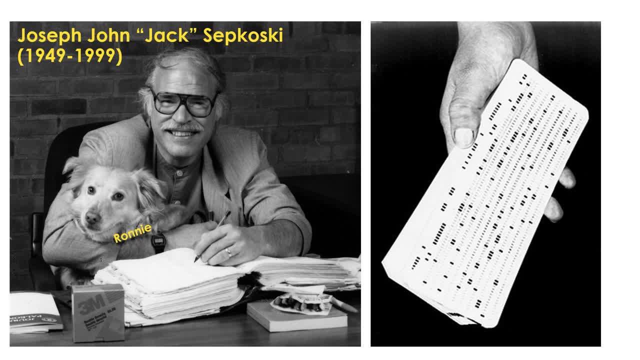 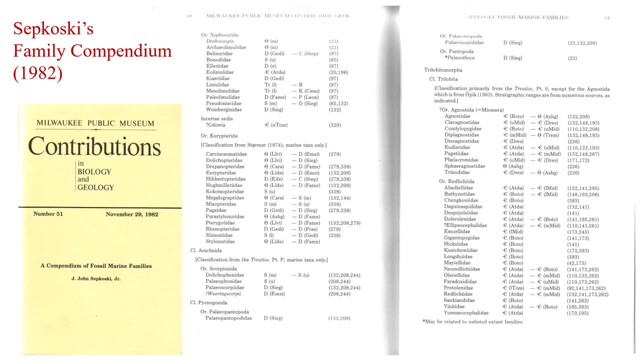 Sapkoski revolutionized our understanding of biodiversity and provided some of the best evidence up until then for the existence of mass extinctions. As a graduate student at Harvard, Sapkoski conducted an extensive review of books and articles in the library and compiled a compendium of 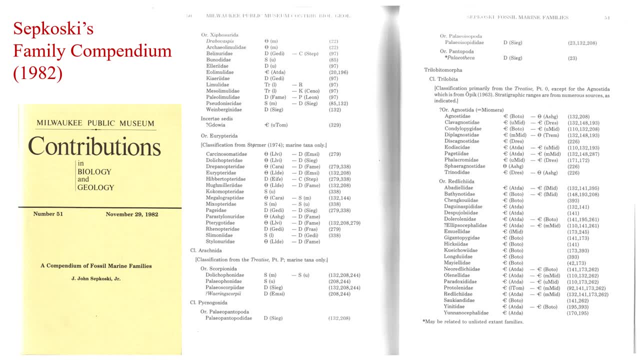 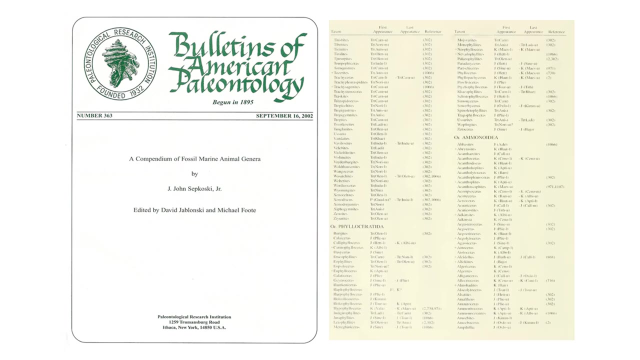 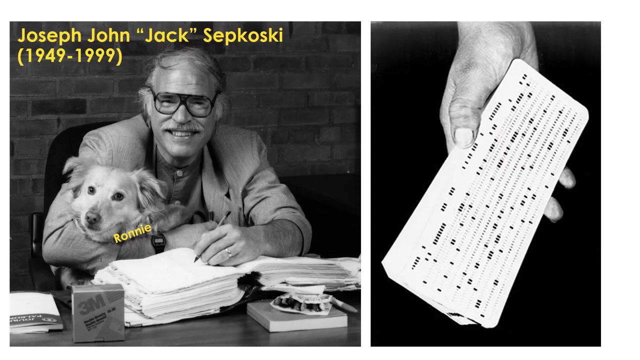 data on thousands and thousands of marine animal taxa, including orders, families, genera and species. the compendium includes information on when each taxon appeared and disappeared in earth history. in other words, it contains information on when each taxon originated and when it went extinct. to facilitate this work, sepkoski compiled the data. 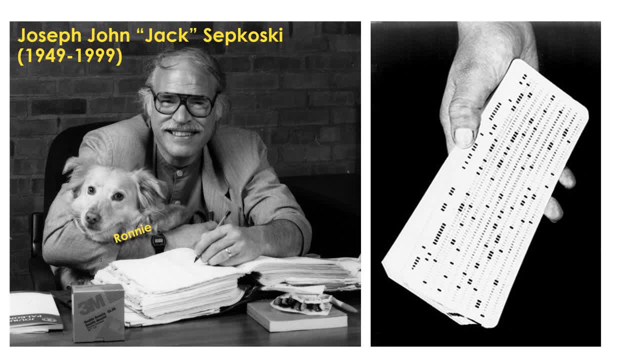 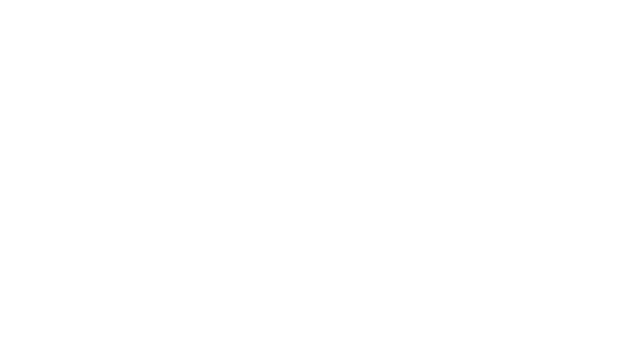 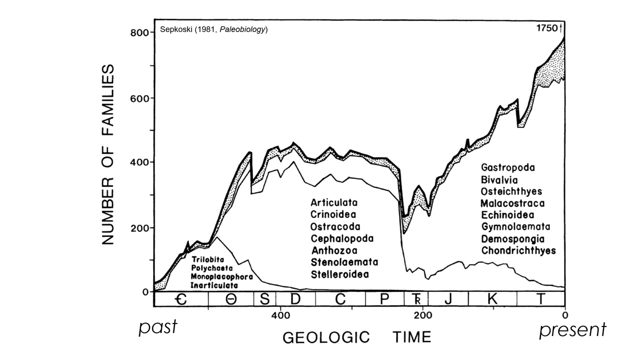 by punching holes in cards, which he fed into the computers available to him at the time. this work took years, over which time sepkoski spent many long hours in the library, but in the end the work paid off. using his compendium, he produced a. 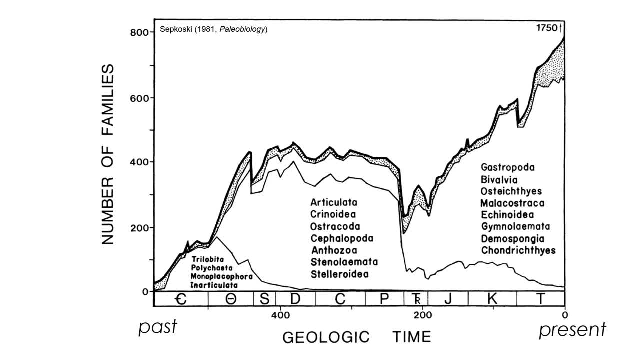 fanner's diversity curve like this one again. biodiversity is represented by the number of taxa. the vertical axis shows the number of families of marine animals preserved in the fossil record. the horizontal axis illustrates geologic time spanning from the beginning of the phanerozoic, 541 million years ago, to the present. 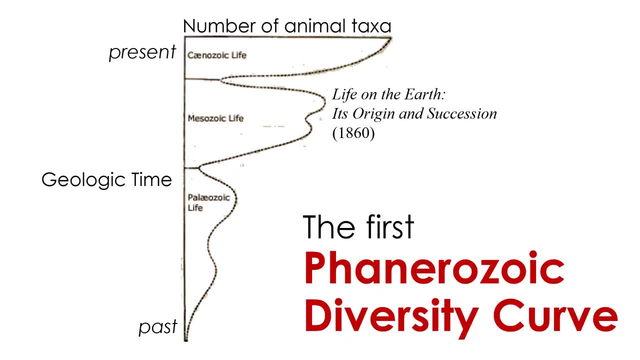 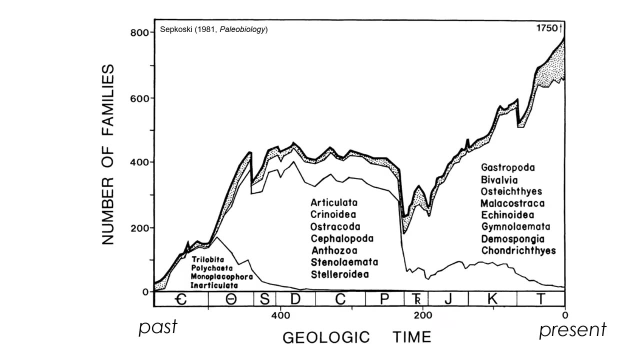 like the diversity curve that john phillips had produced more than a century earlier. sepkoski's curve showed that the number of taxa has increased over time. the biodiversity of the planet has grown over the past 541 million years. in addition, sepkoski's work revealed two other interesting trends. 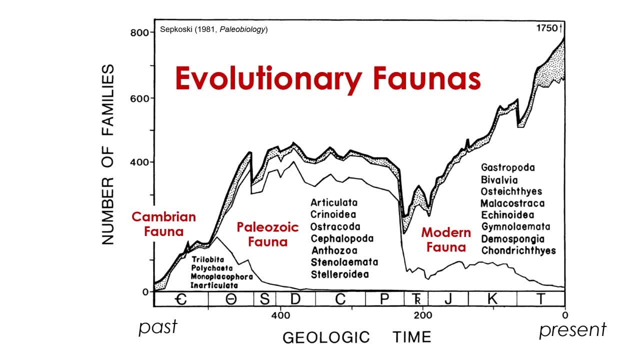 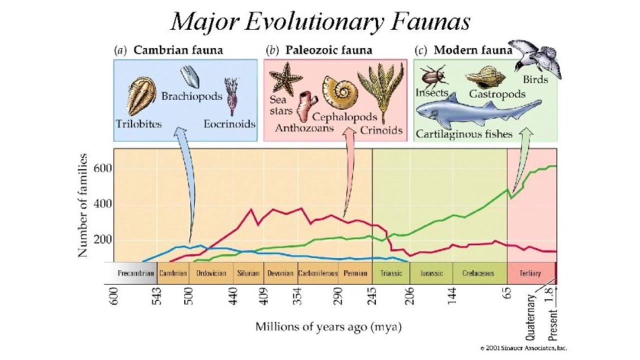 first, he showed that there were three groups of marine animal taxa that rose to prominence and declined in unison. each of these groups, which we call evolutionary faunas, dominated a specific time interval in terms of number of taxa. the cambrian evolutionary fauna consisted of trilobites, inarticulate brachypods and worms that. 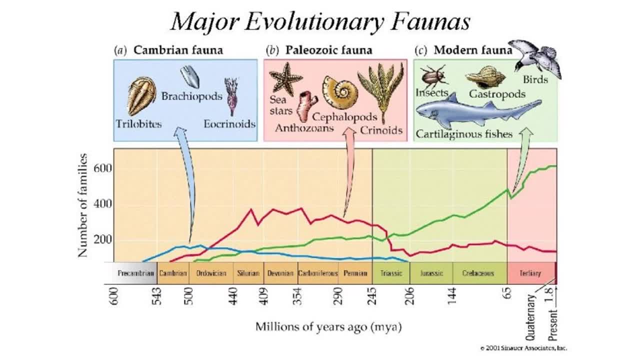 were very diverse. in the cambrian in the paleozoic, most taxa belonged to an evolutionary fauna consisting of articulate brachypods, cryonoids, cephalopods and coral, among other things. finally, the modern evolutionary fauna dominated the world in the mesozoic and cenozoic. 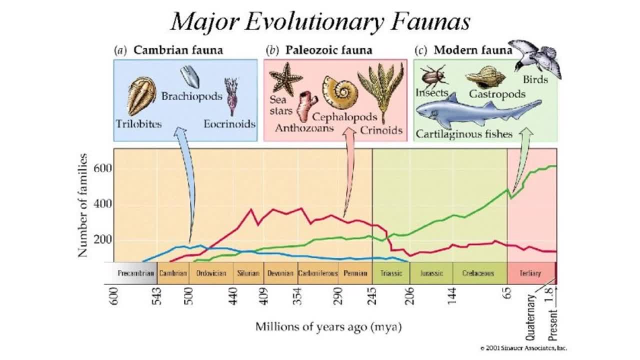 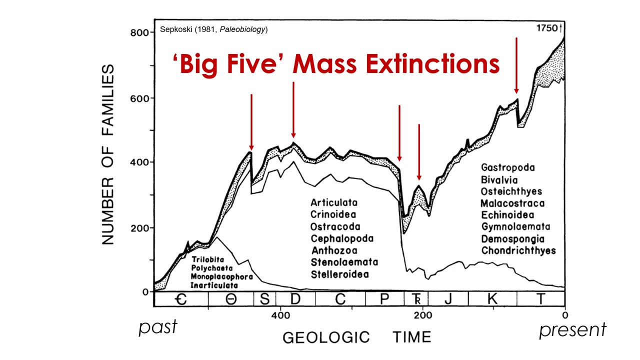 it still dominates the world to this day, with most marine animals being snails, clams, crustaceans, fish, shark and sponges. most importantly, sepkoski's work demonstrated that there were five times during the phanerozoic eon when the number of taxa sharply and significantly dropped for a time. 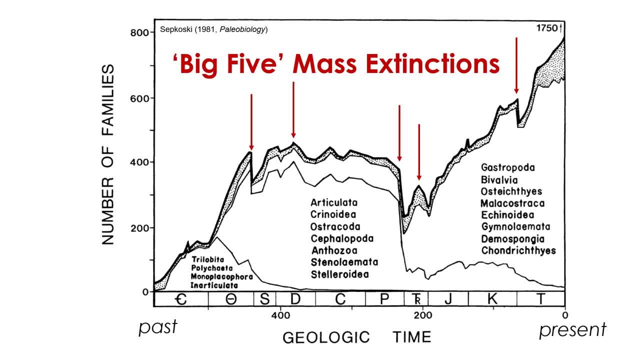 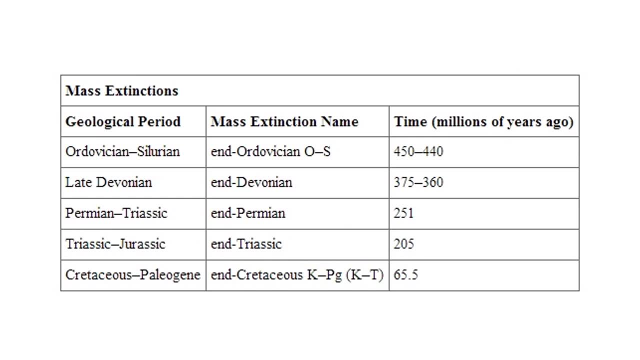 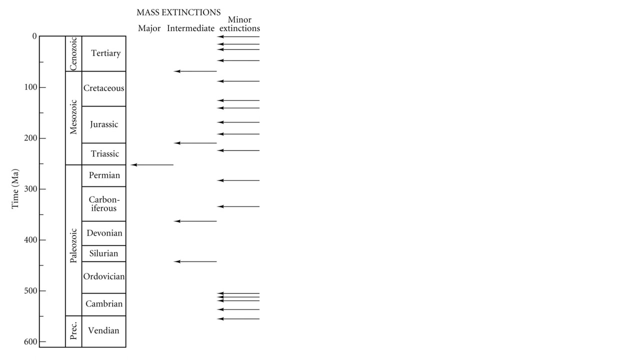 these drops represent rapid declines in biodiversity caused by the extinction of taxa. we now call these events the big five mass extinctions. these mass extinctions occurred at the ends of the ordovician, devonian, permian, triassic and cretaceous periods. there are other extinction events in the last 500 million years, extinction events of minor and. 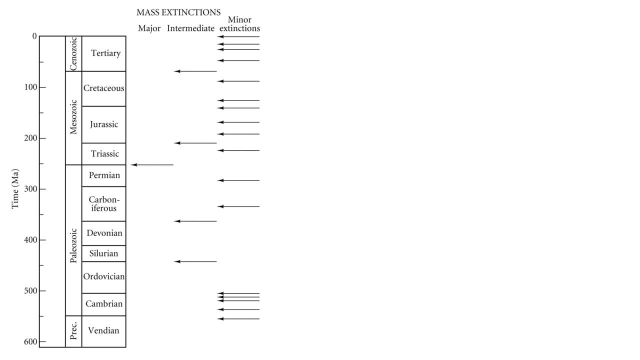 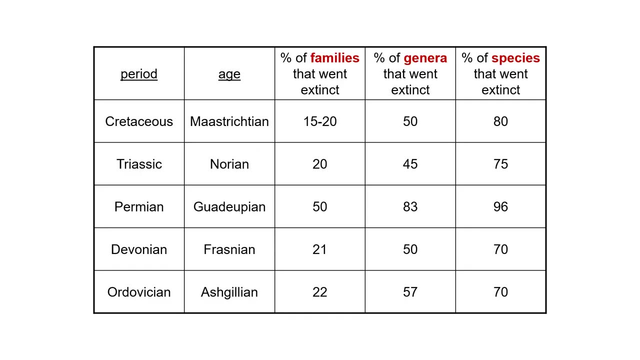 intermediate scale, but the big five were by far the largest and the most severe extinctions. the permian mass extinction was the biggest. some estimates suggest that 96 percent of all species on earth went extinct at that time, around 251 million years ago. the other mass extinctions likewise saw the disappearance.